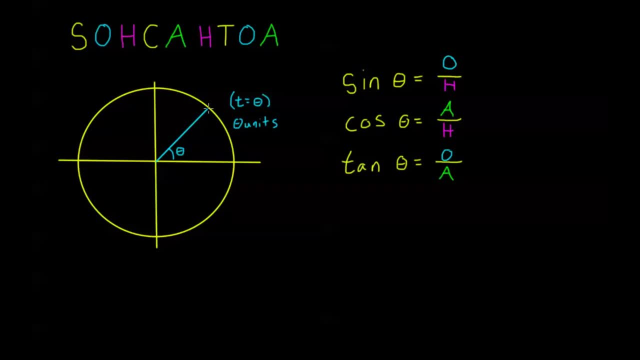 So I'm going to go ahead and bring this line down from this point on my unit circle straight down to the x-axis, right here, All right now. we see this. We see that that forms a right angle between this line of this triangle and the x-axis. 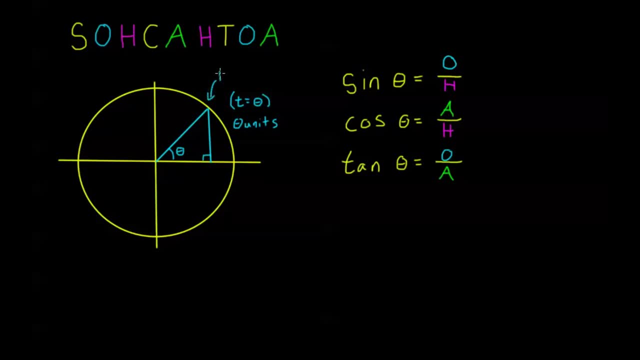 Now, if this point up here is my terminal point, Pxy, determined by either my real number, t, or my radian angle, theta, we see that it's the same point, determined by both right, And the measurement is the same, even though it's in different units. 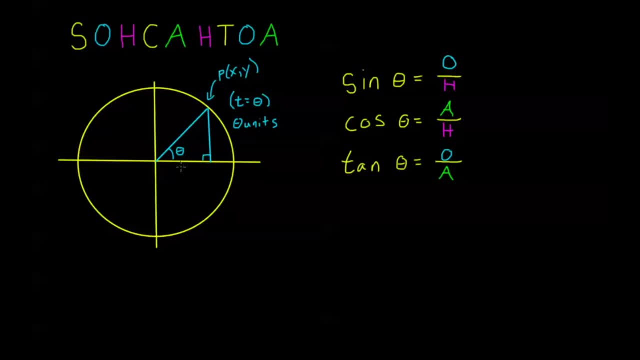 I have that this side of my triangle is going to be equal to x. whatever, the x of my terminal point is right. I've come straight down, I've come straight up from there and up here we see that this is equal to y. 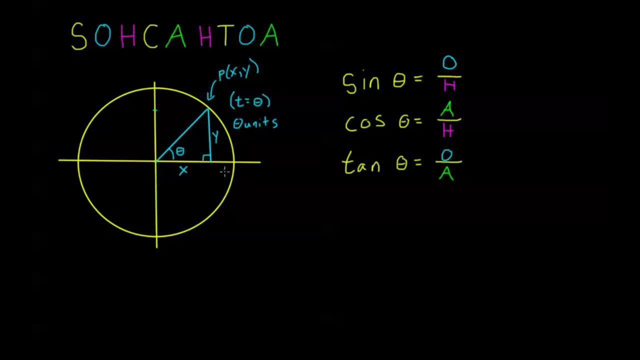 So this, the whole length of this side of my triangle, is going to be equal to y. So let's go ahead and define our sine, cosine and tangent just based on this. We see that from SOHCAHTOA, my sine of theta, theta, the real number right on the outside, my real number, theta, by SOHCAHTOA. 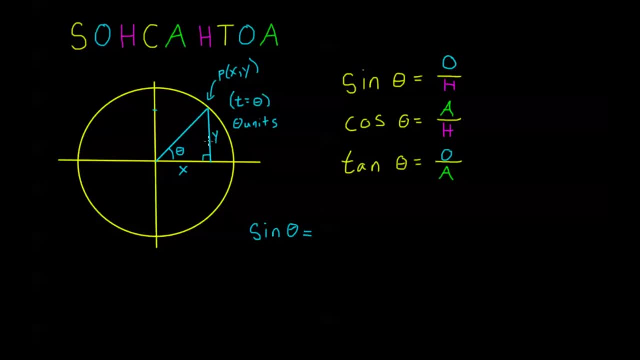 So of course, we're going to use SOHCAHTOA And this is going to be equal to my angle theta, That's equal to my opposite over my hypotenuse. Now, I didn't do this part yet. We're on my unit circle. 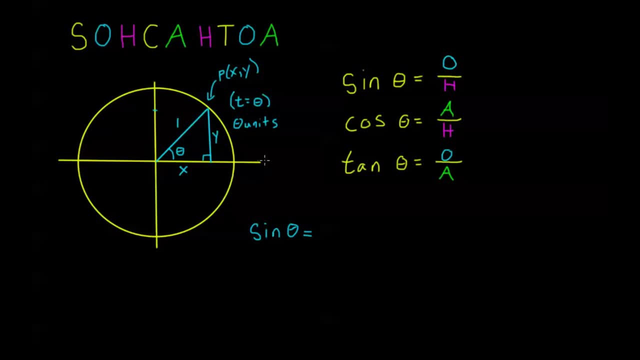 So, of course, this hypotenuse has a measurement of 1,, doesn't it? So sine's going to be equal to my opposite side over my hypotenuse, which is y over 1, or in other words y. 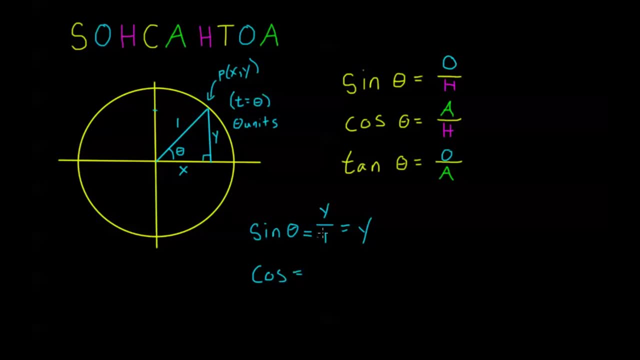 Cosine. this is going to be equal to the adjacent side of my right triangle over my hypotenuse, or in other words, x over 1, or just x and tangent, leaving out my thetas, again tangent of theta. this is going to be equal to my opposite side over my adjacent side. 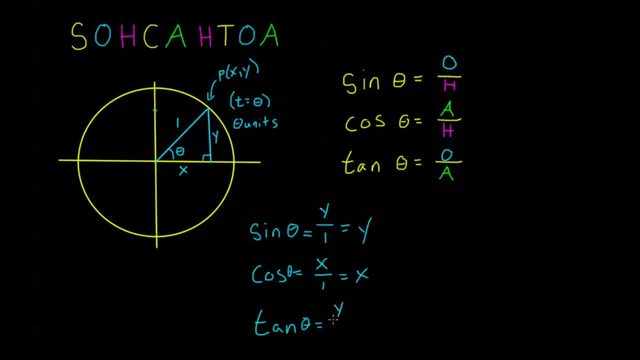 so, in other words, y over x and no simplification necessary here. Now, if you go back to our real number section, when we define these trigonometric functions, these are the exact definitions that we gave, based on the real number around the circle, and we can see that sine of theta. in other words, let's say that: